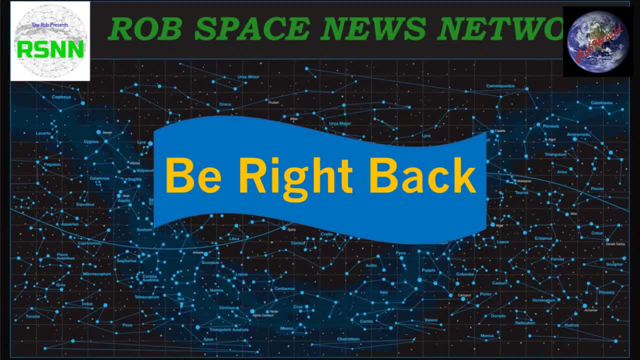 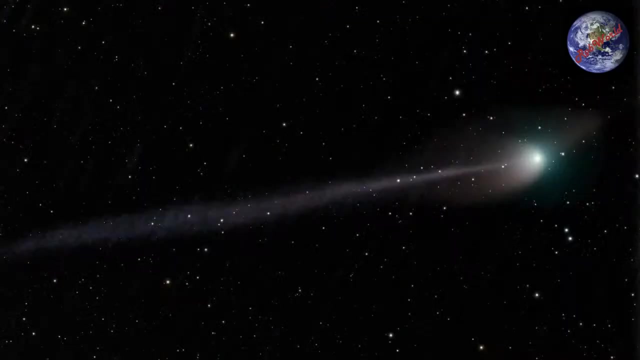 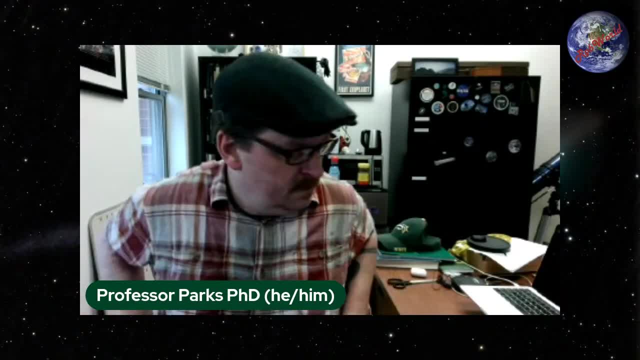 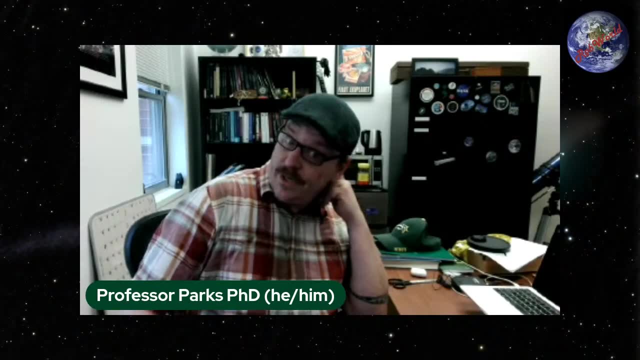 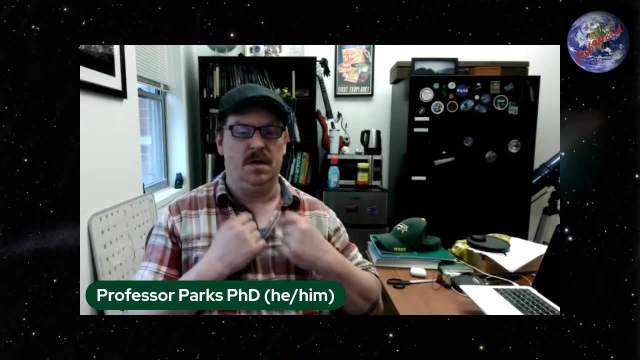 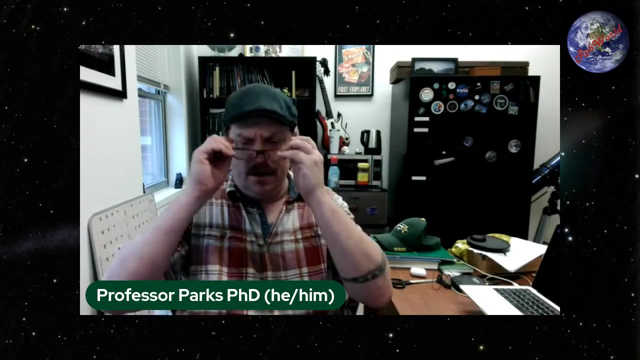 All right, That'll do it, boys. Okay, Whew. um. so i just recorded a lecture um in my office, which is way, way too hot, so if you don't mind me getting a little sexy for you. um, yeah, it went way longer than i anticipated. um, and yeah, hot. 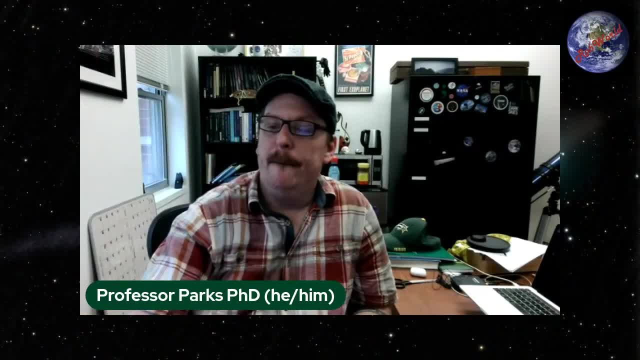 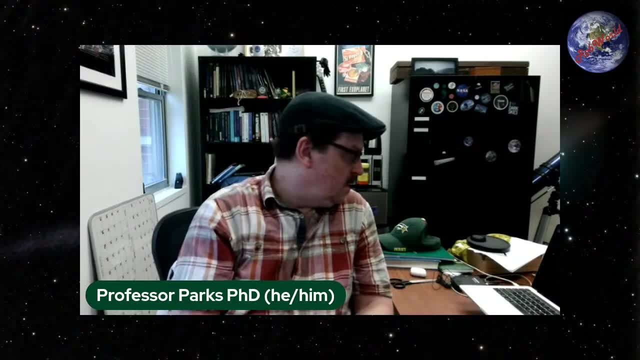 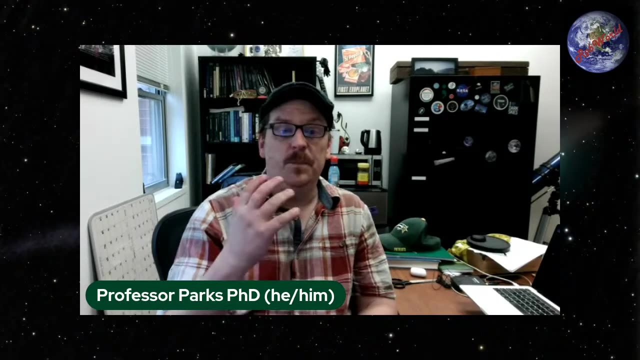 sweaty anyway, hot and bothered, i guess. uh, the lecture, if you were wondering, which i'm going to be posting right after this um is hopefully is not too terribly long. i actually don't know how, how old or how long it is. uh, it's about, um, how to use galileo's incline incline plane experiment. 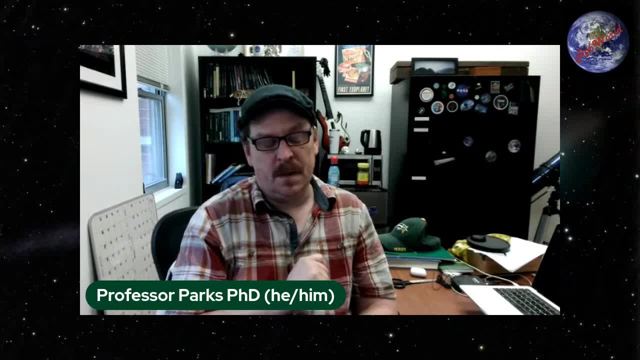 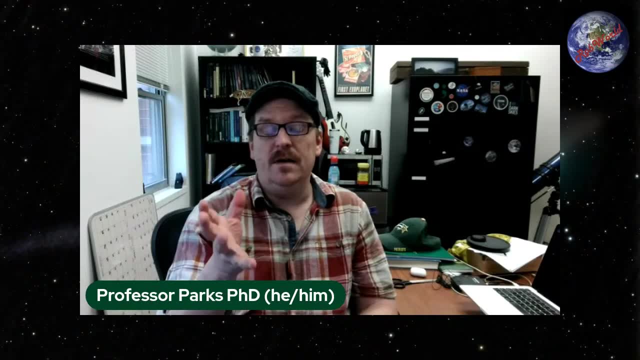 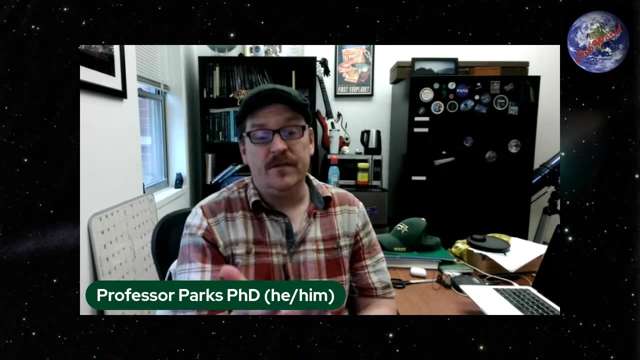 to demonstrate that gravity is a thing. um, and it's later i i latched on to the idea that this is an awesome way of just talking about the scientific method, how science is actually done, and so hopefully folks will enjoy it. um, it probably should be edited. there are a few times when i uh, 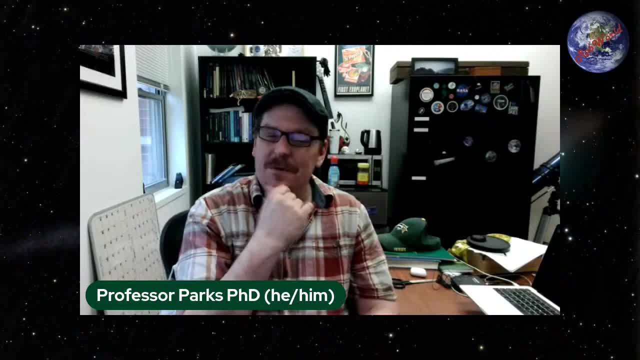 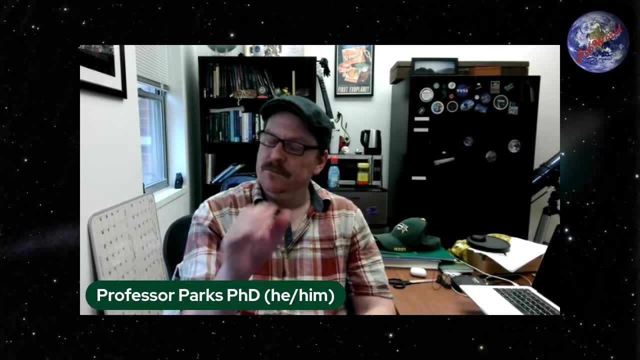 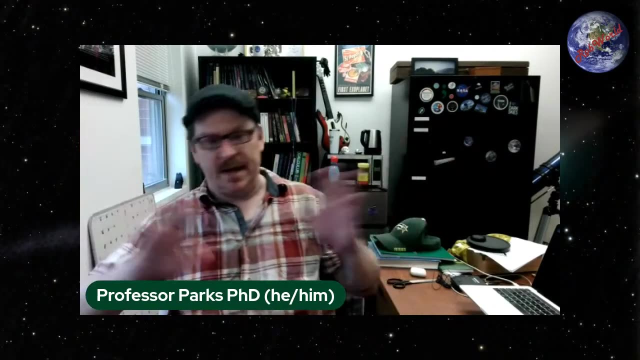 um, i i stumble on some things, so shall we say, but i think ultimately it's all right, it's all good. um, if it isn't, i trust uh folks to let me know. but anyway, anyway, that's neither here nor there. howdy nimrod, uh, clive judy. 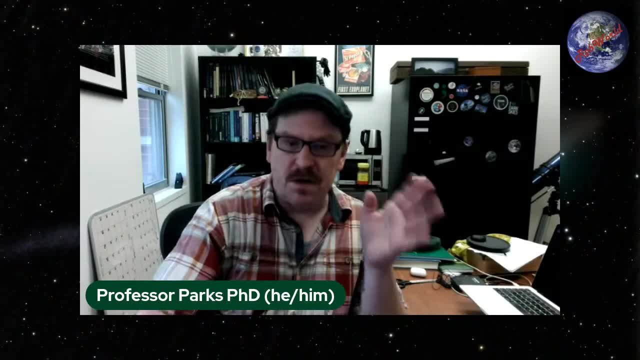 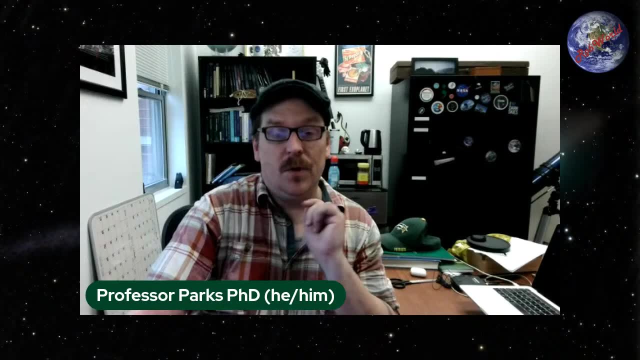 how are you? um, that is neither here nor there. what we're talking about today, what we're here today to talk about, hey, gay, or is not what i said we were going to be talking about at the end of the last lecture? the end of the last lecture, i said we were going to be talking. 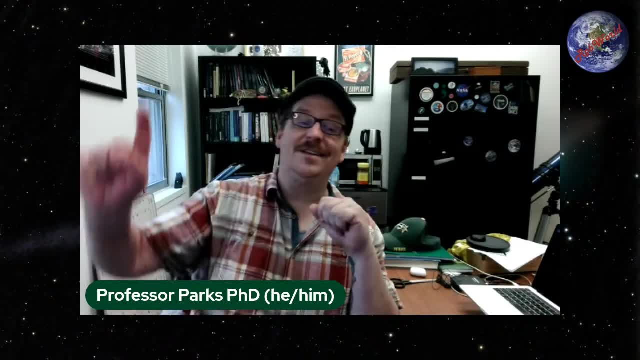 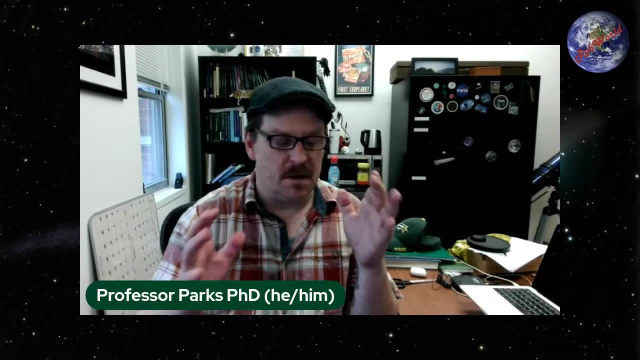 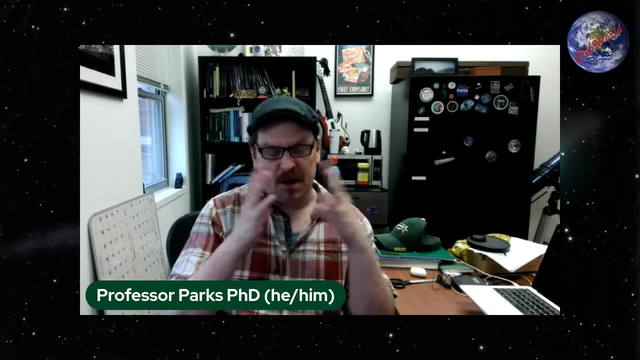 about the sun. when i checked my schedule, actually, the sun is up and i'm going to be talking about it. the sun is at the end of the semester, So I'm going to be starting to talk about planetary geology. I'm going to start off with talking about, well, planetary geology. I'm going 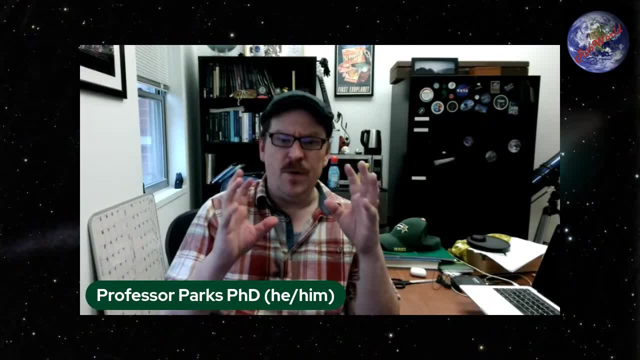 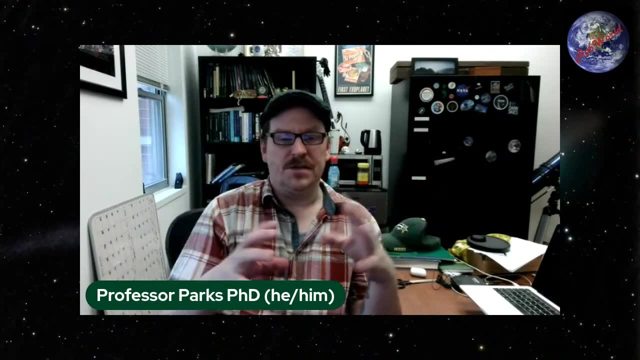 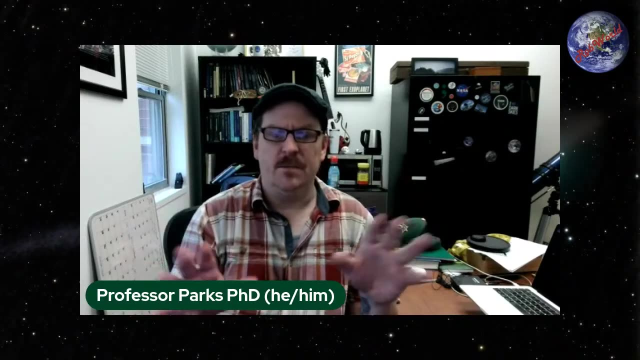 to be talking about a couple of different methods on how we know what we know, or you know, you've seen those, you've probably run across those models or pictures of the earth where you have the core and the outer core and the mantle and the crust and all that. 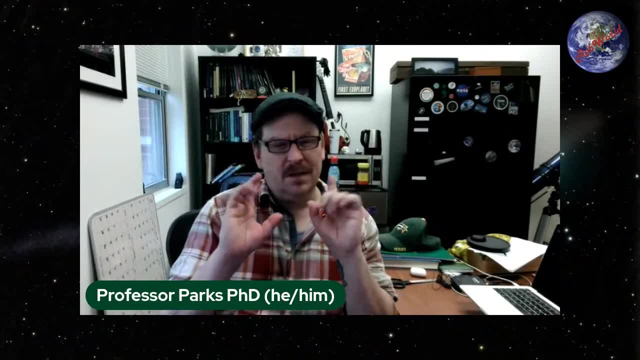 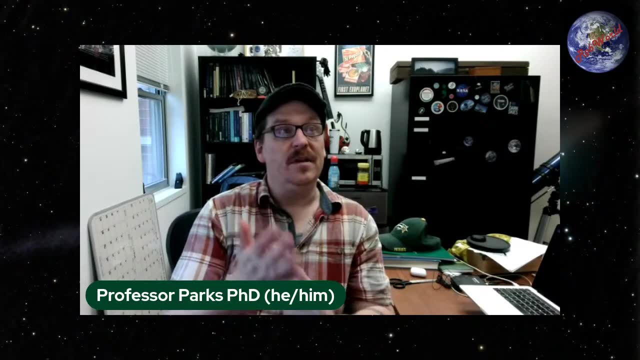 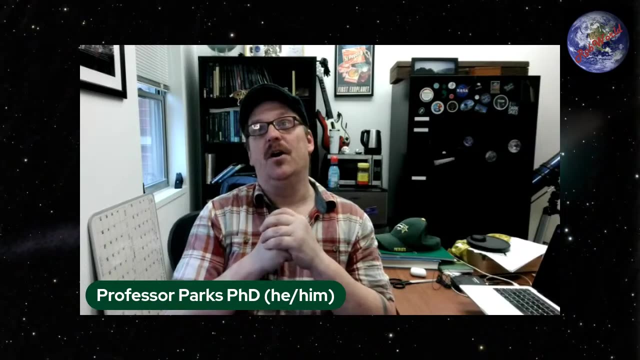 kind of business. We'll talk about a little bit on how that model is created. Now, I am an astronomer, not a geologist, So I will. I am going to be really hand wavy about it because my geologist friend tells me that he hates that diagram because it is an oversimplification. 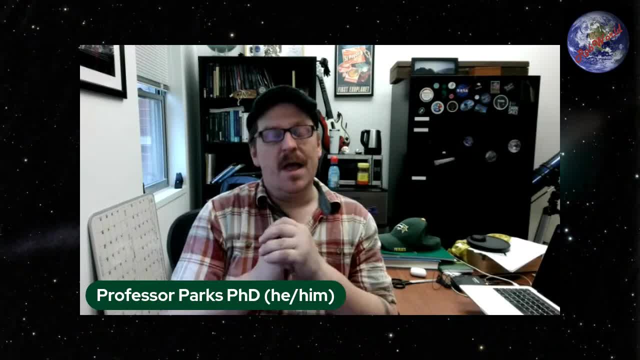 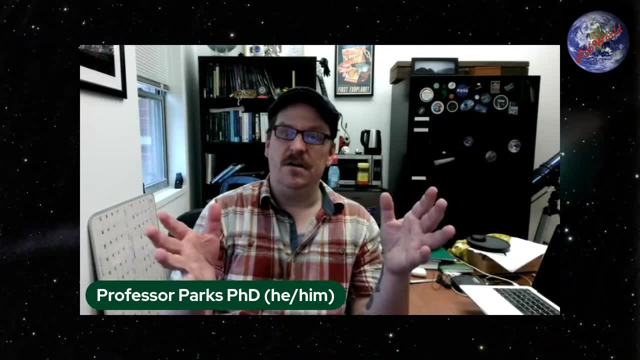 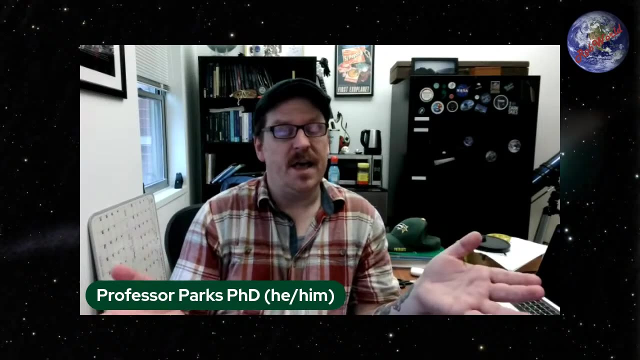 of the complexity of the earth's interior And I'm going to relate how. that interior is very similar, we believe, to the interiors of the other three terrestrial worlds, And I will talk about why. why that is? How is it that those that those worlds came into? 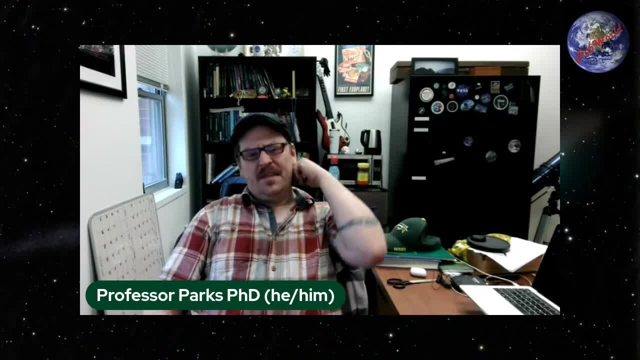 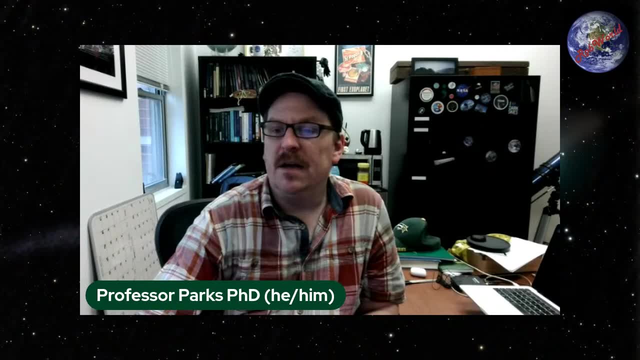 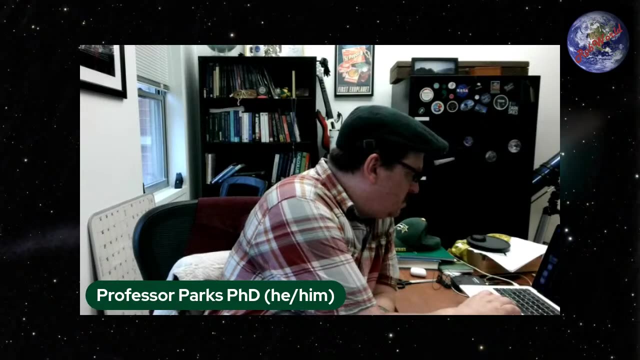 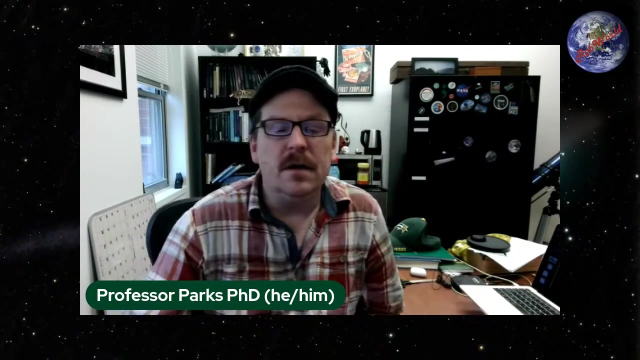 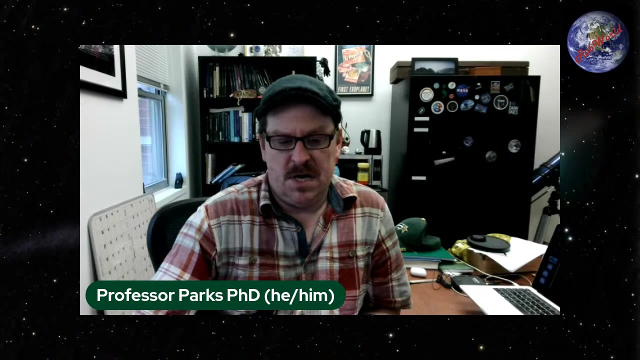 being like that. Ah, Indy, I think I mentioned you in my last lecture. How are you All right? Like I said, I am a bit late. Let me do this. I'm going to make sure that it's saved. Yes, vertical is on. I don't care. Present Slides. 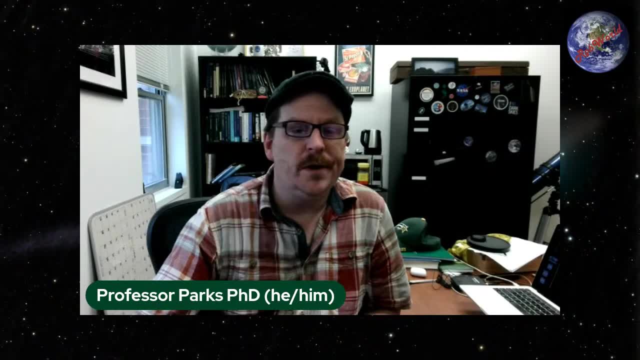 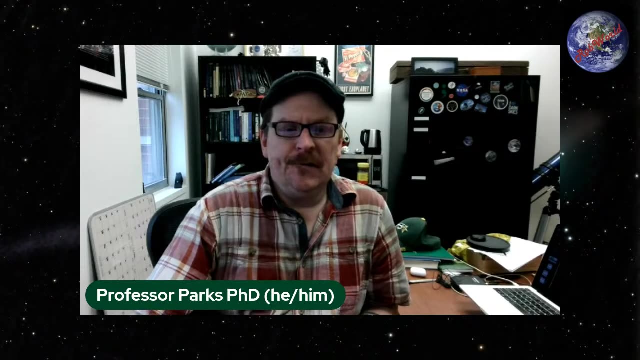 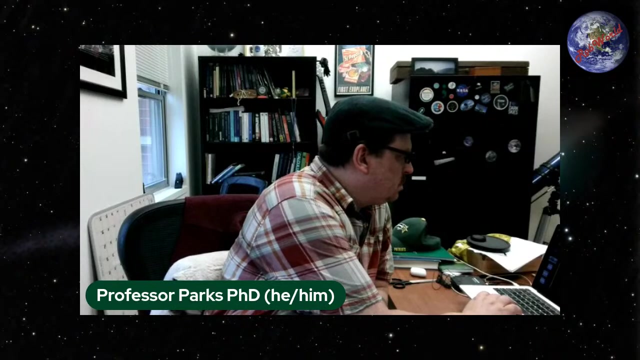 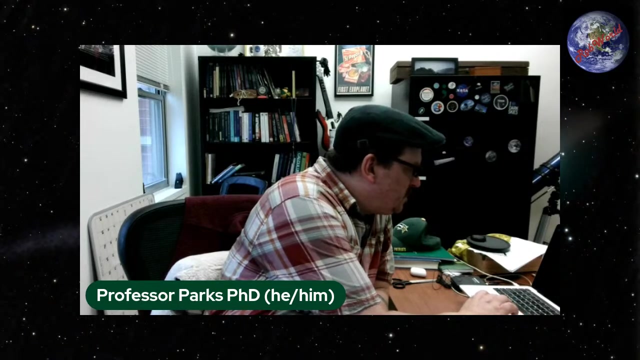 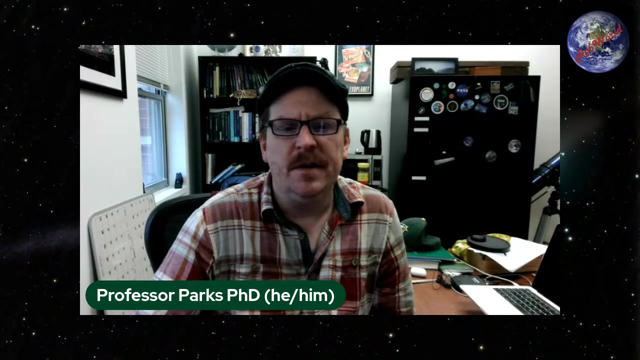 Computer Man, I am dehydrated. Ah, Oh, Huh. Why did I save this? Ah Darn it. Hmm, I can't seem to find it. Hmm, Hmm, Hmm, I can't find it. 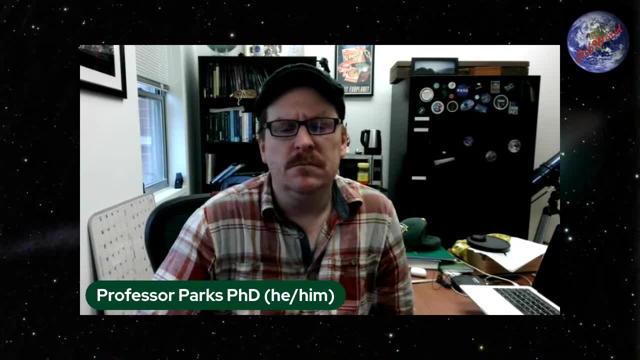 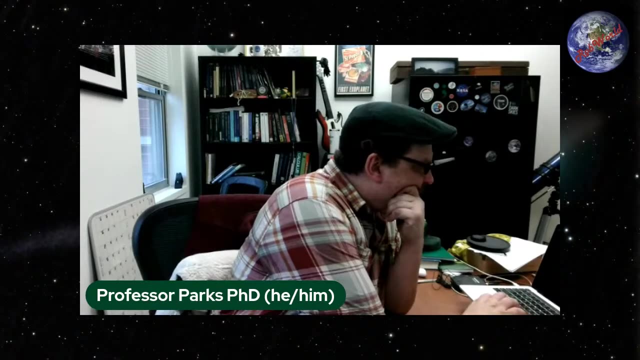 Well, that is annoying And I can't seem to see it on this, because Zoom is converting my- uh, Zoom is converting my lecture at the moment And so I can't have. I don't have access to why my microphone is not working. 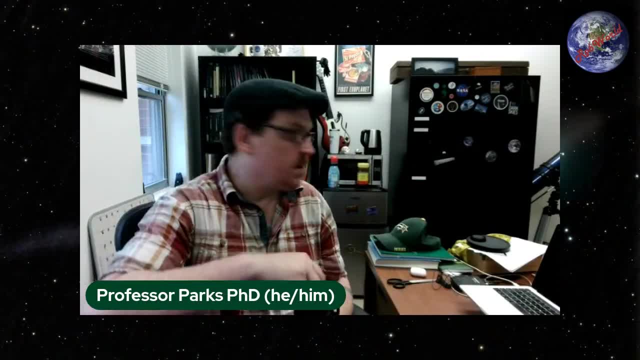 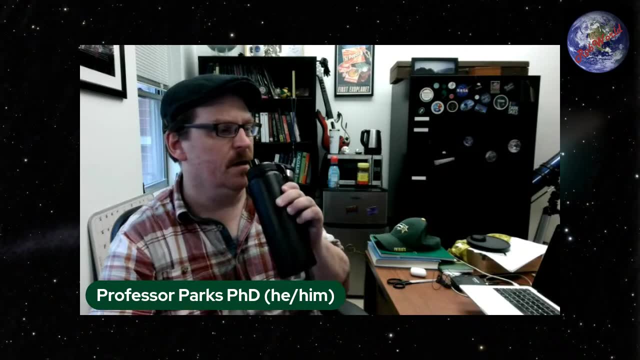 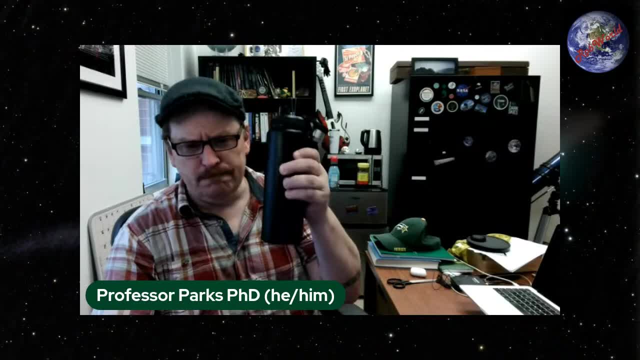 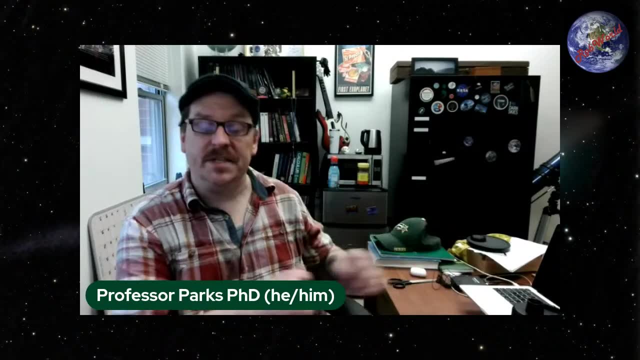 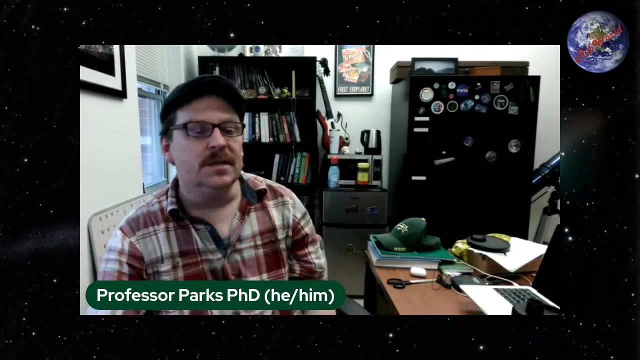 Thank you, Nimrod. I am going to drink lots and lots of water. So all that's doing its thing, And while I uh show how professional I am and you know uh doing my stuff, uh, let's. 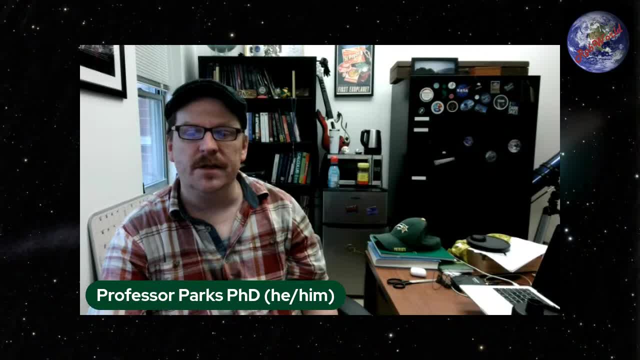 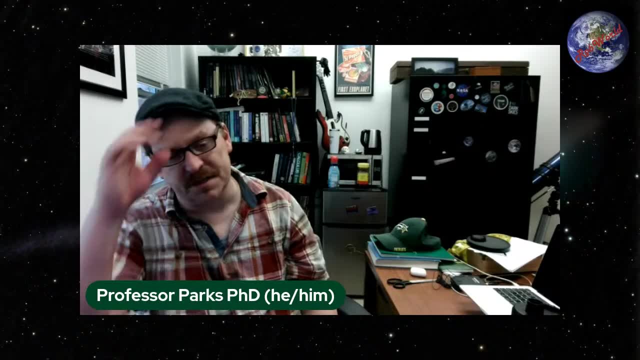 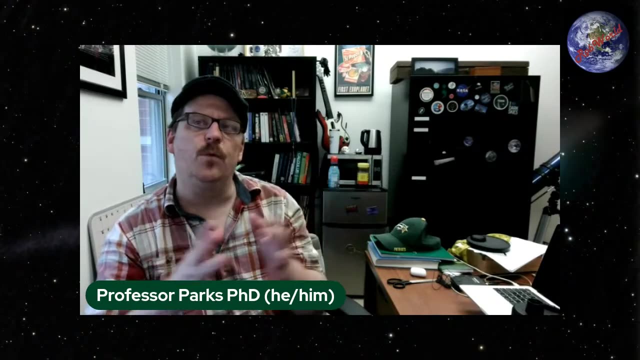 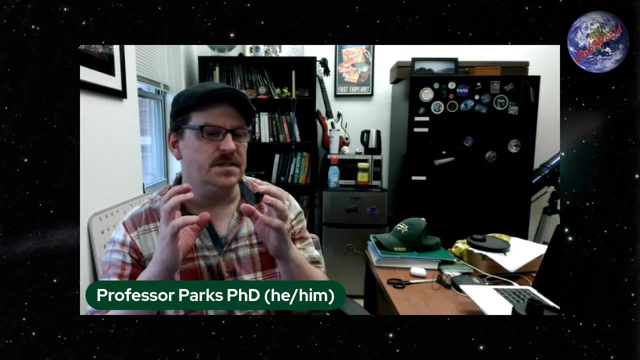 talk about? um, yeah there, Oh Yeah, I was actually in a colloquium. I was listening to someone's idea of they were putting. basically the idea was they wanted to know what were the constituent factors for why Starlink satellites deorbited February 2nd of last year, February 4th of last year. 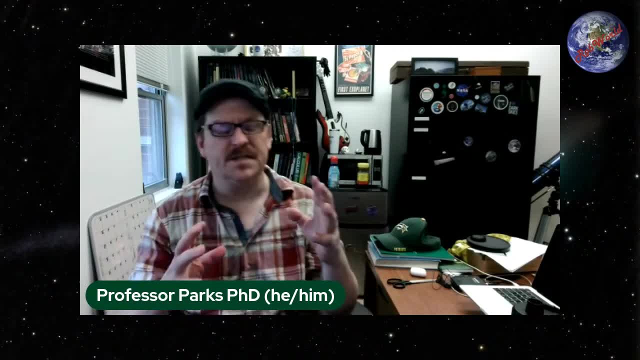 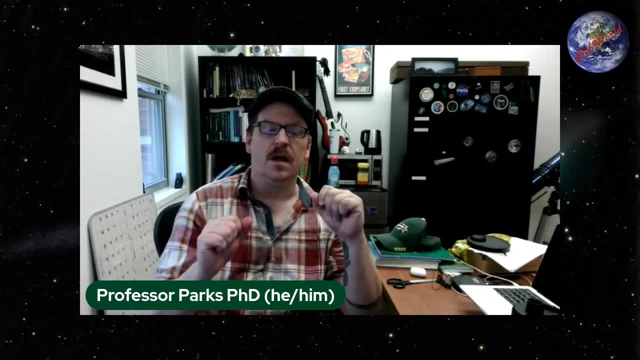 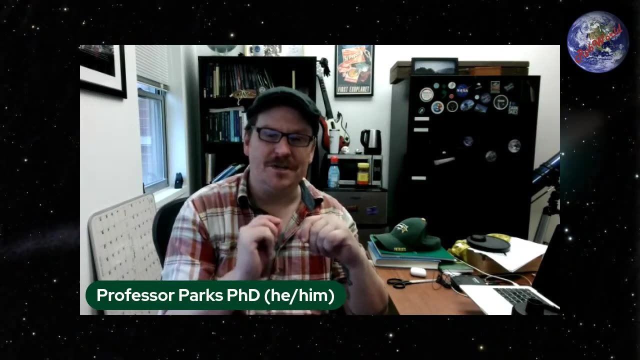 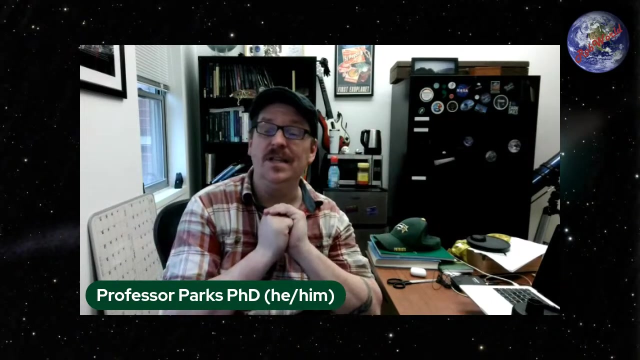 If you don't know, Starlink puts up their satellites in chunks of- in this case, I think it was 48. I heard that they were doing chunks of- no, I'm sorry, They do do it in chunks of 14 or they do do it in chunks of 60- and 48 of them basically crashed into the atmosphere and burnt up and made a really really pretty light show over Puerto Rico. 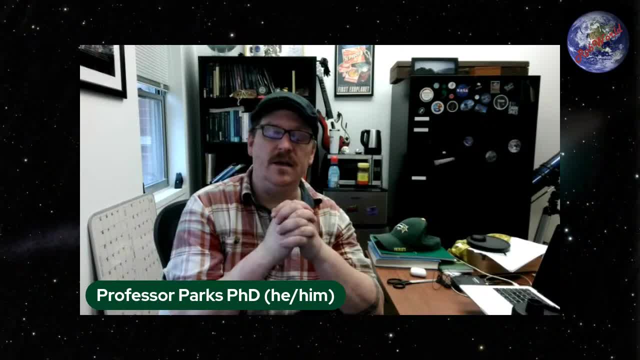 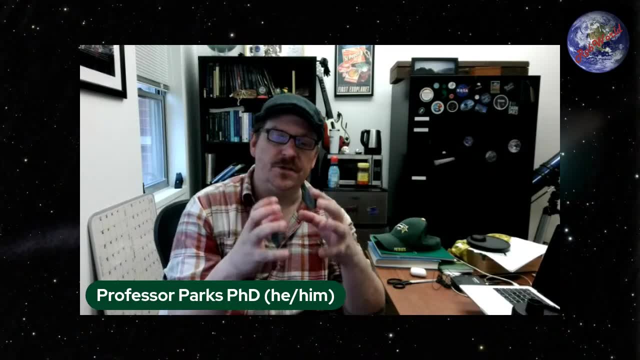 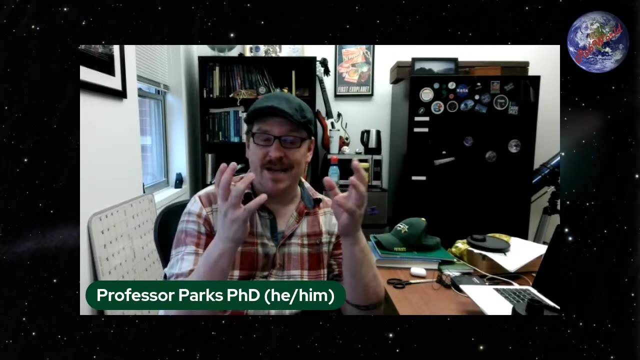 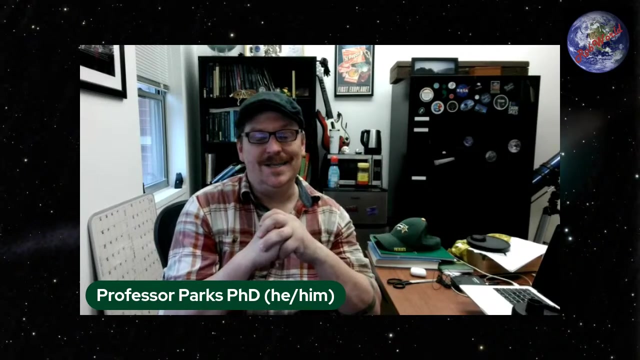 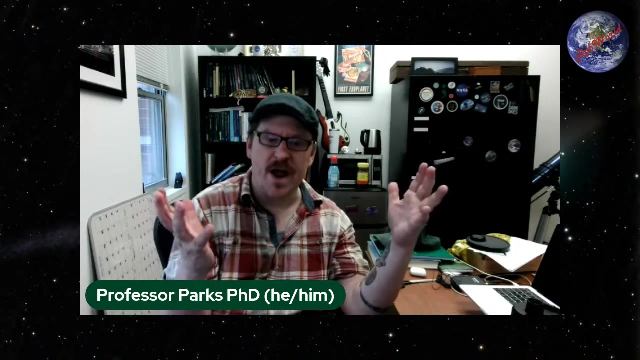 And so this gentleman was Putting forward a model to try to differentiate how much of the cause of that was due to geomagnetic, storm or solar irradiance, Basically the sun's activity heating up the atmosphere and causing essentially the number of neutral oxygen atoms to increase and therefore cause more drag. 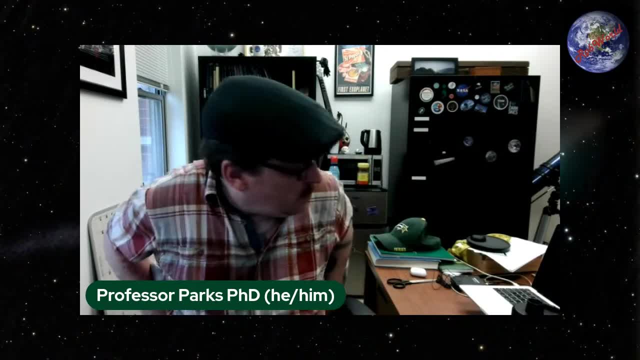 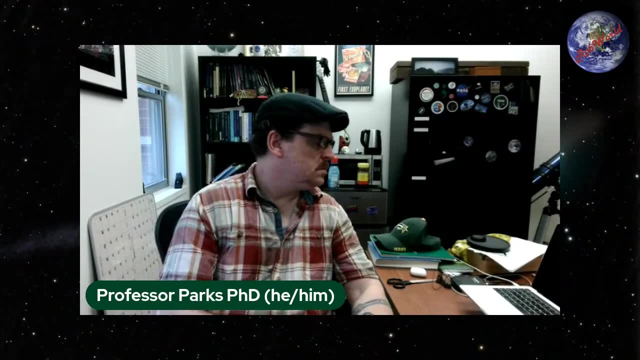 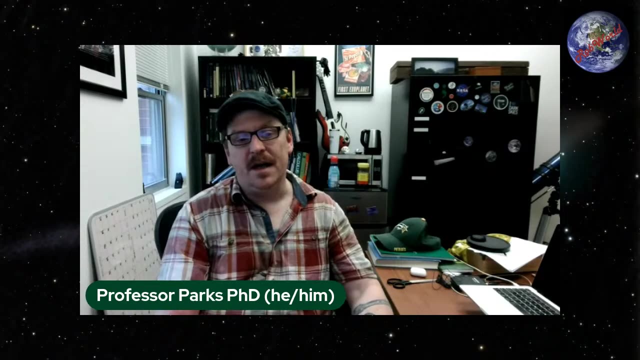 And So so forth and so on, And the orbit stuff Almost there. It says it's there. So yeah, that was really. that was a. so yeah, I was. unfortunately I missed Eddie's, Eddie's thing. 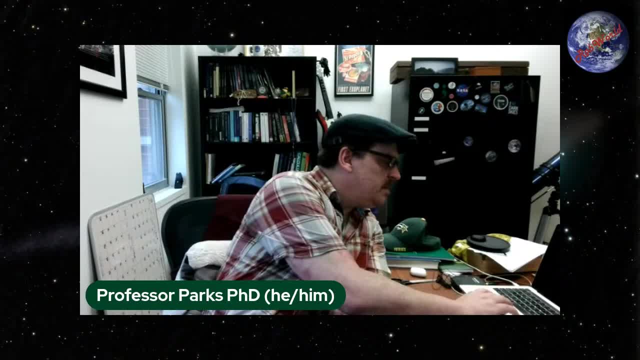 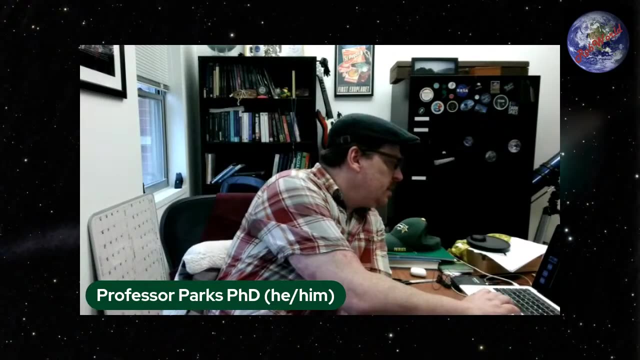 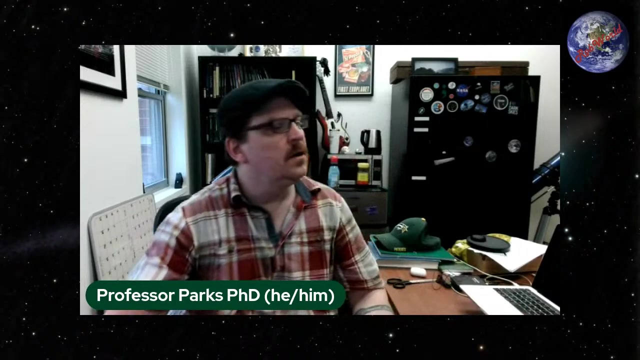 And I haven't talked to. I haven't talked to Crafty in a while. Let's get back to this. I'd like to replace it. All right, I want to make sure I actually have this right. This is saved in courses. 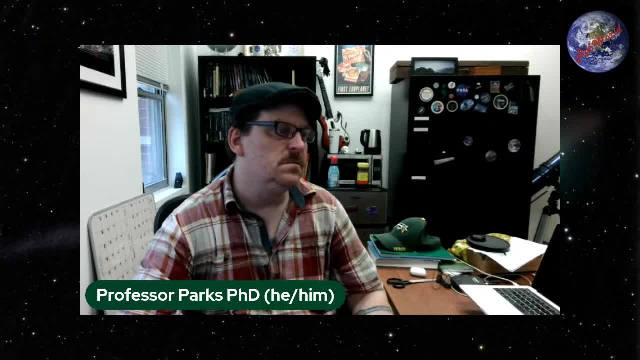 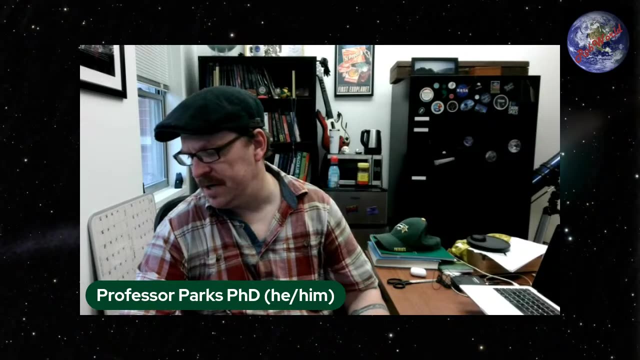 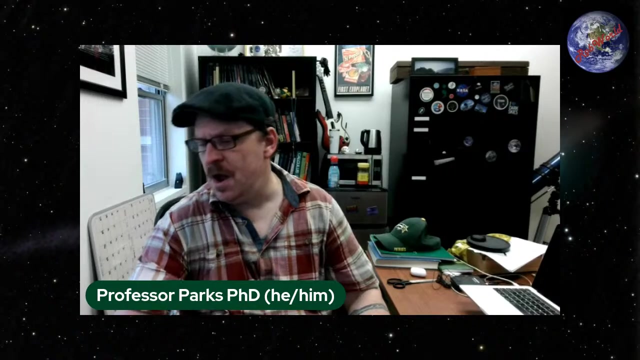 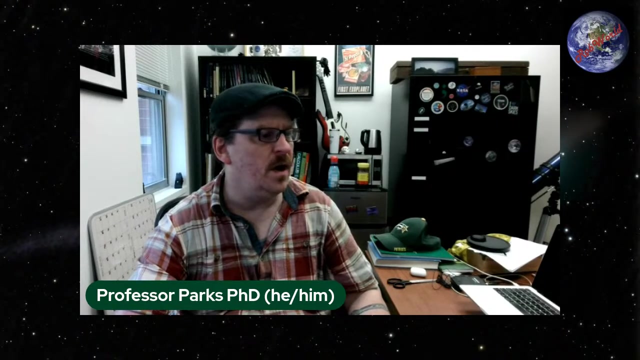 Spring 2011.. All files. What the fudge, What the hey. why aren't you updating Dropbox? No, No, Why, Why are you doing this to me? I truly apologize for this, guys. I'm sorry. 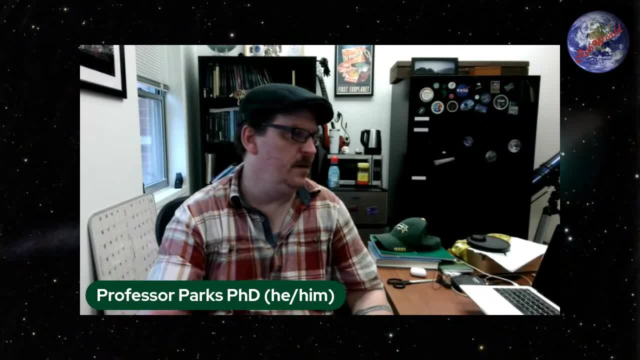 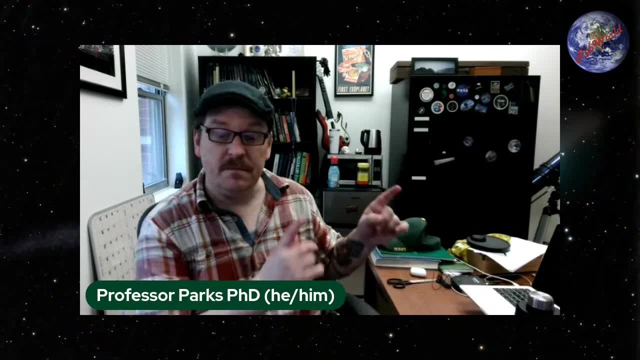 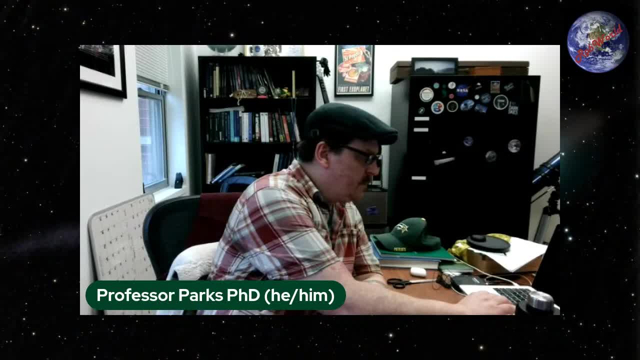 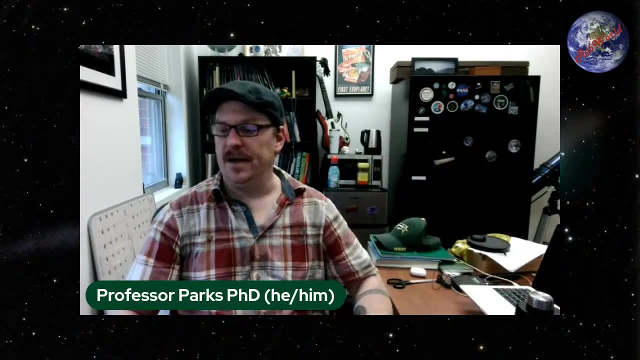 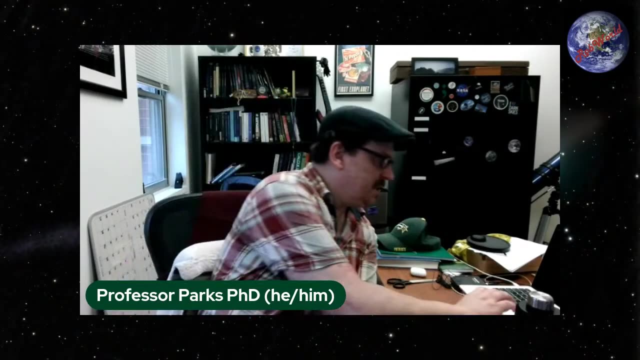 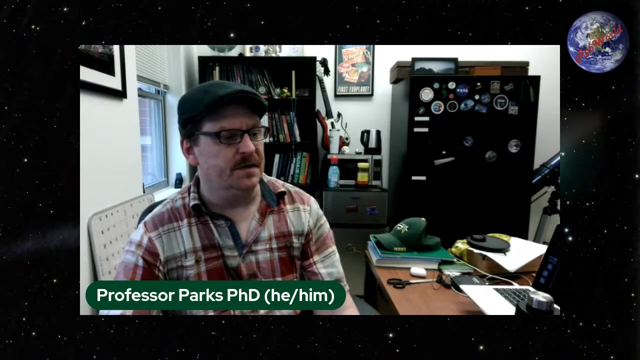 And then I typically save them, Save them to my Dropbox account, which is linked to my Linux box, which is here, And so typically, typically, it's a very kind of instantaneous- Oh Yeah, instantaneous process: I save something here and it goes there. Let me just do this, Nope. 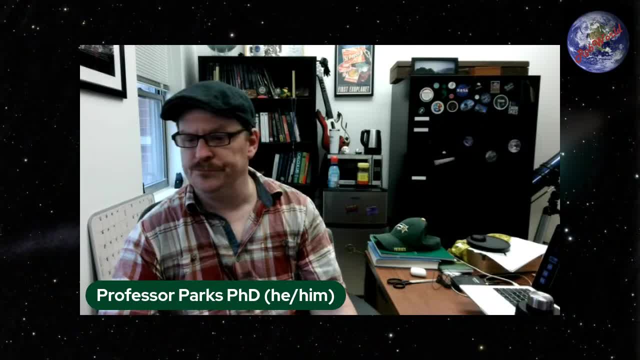 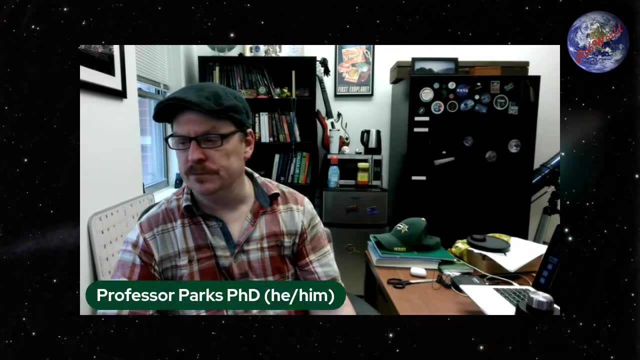 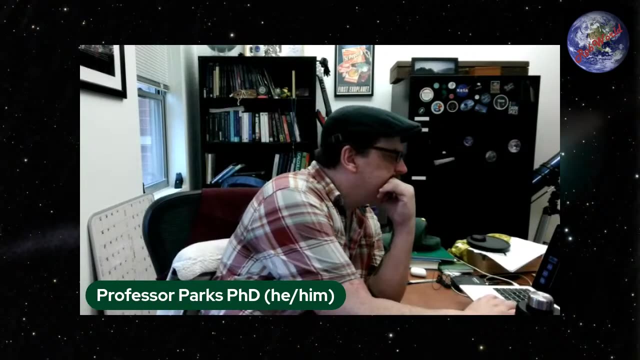 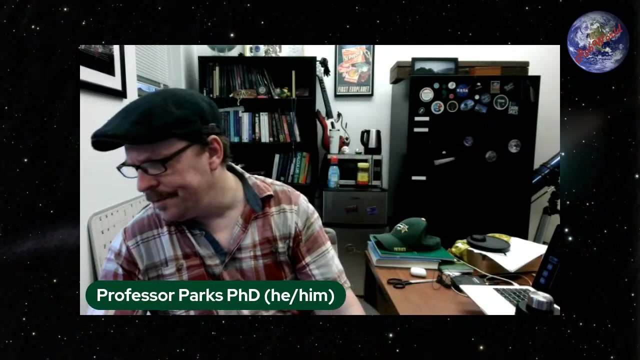 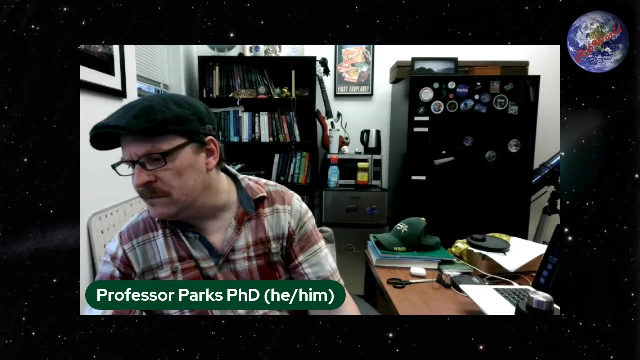 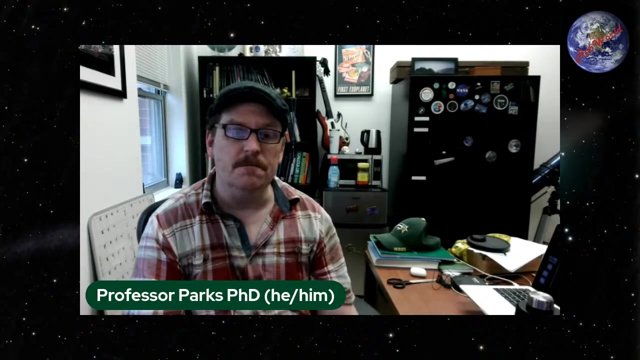 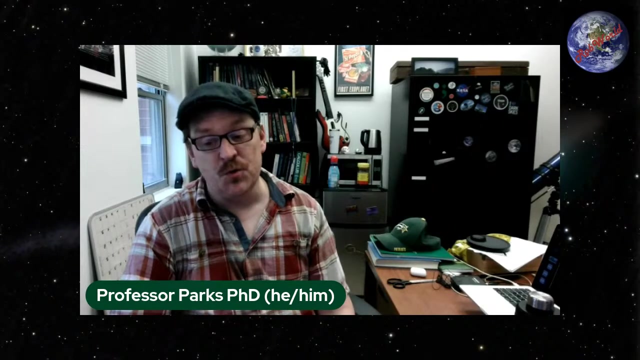 Oh, that's all. That's awesome. All right, folks. I think one might have to do just drop on. No, that's discord. What I might have to do is actually close down this stream and switch over to my Mac, because I know it's on there. So two monocles: I don't even know if I'm cool enough to do.